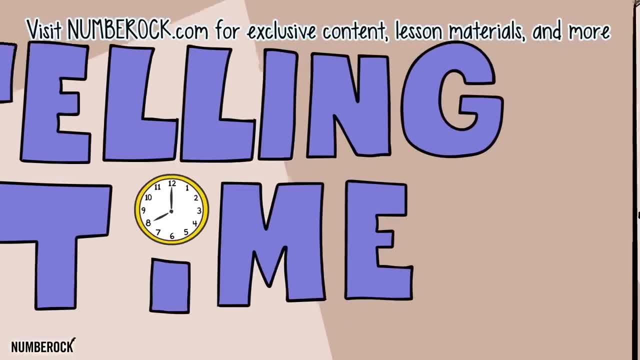 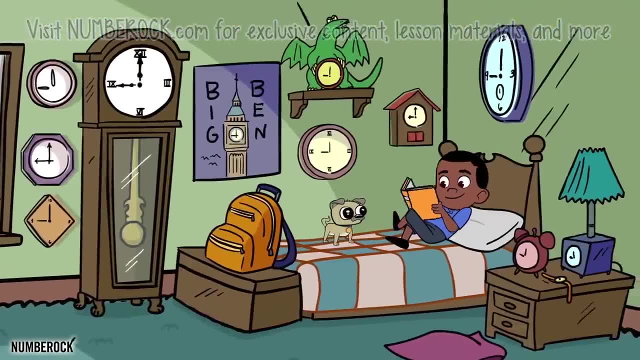 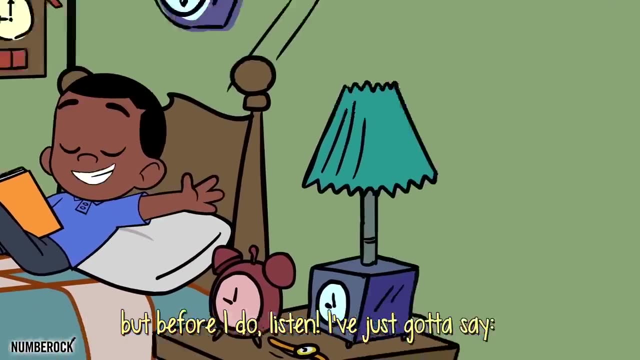 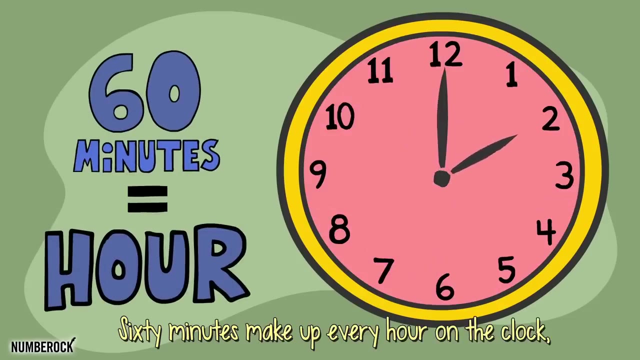 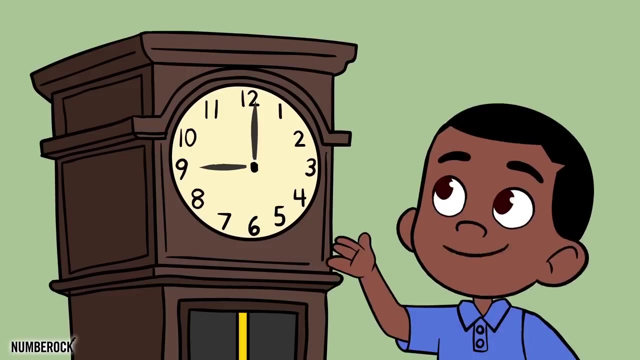 I want to tell you all about my Saturday, but before I do listen, I've just got to say: 60 minutes make up every hour on the clock and every number is five minutes. Tick-tock In 12 groups of five. 60 minutes make an hour. 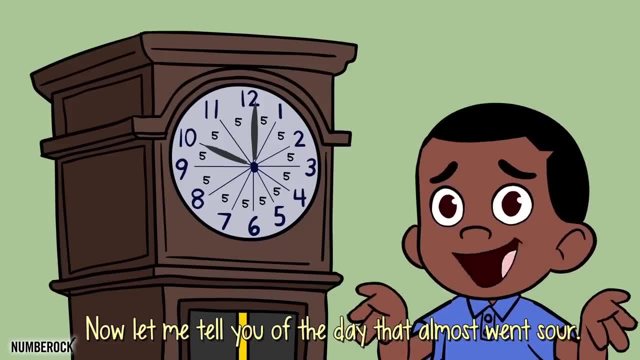 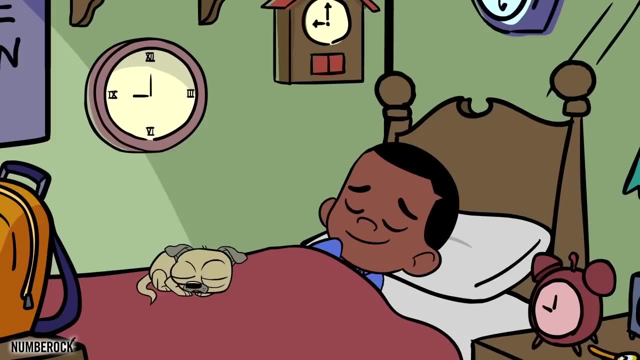 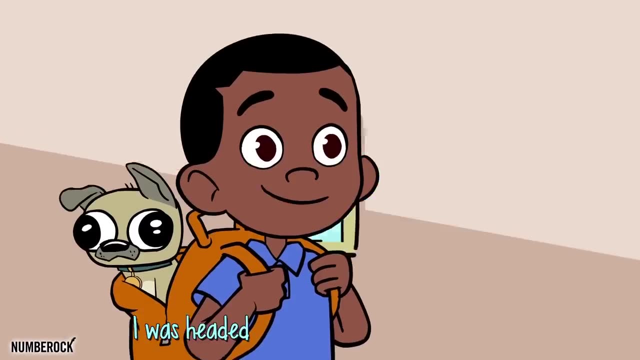 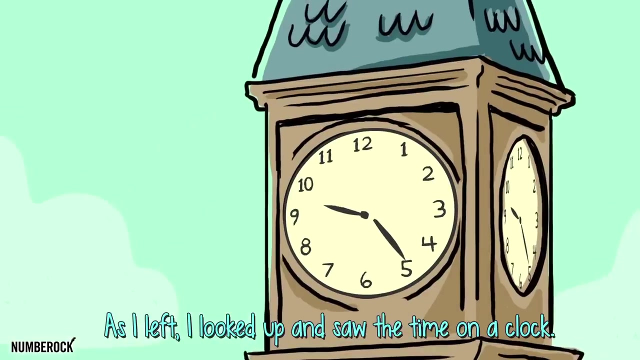 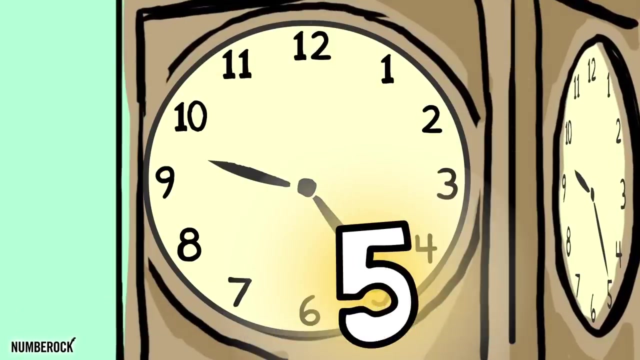 Now let me tell you of the day that almost went sour. Oh yeah, I was headed to the park. I decided to walk As I left. I looked around, I looked up and saw the time on the clock. The shorthand was after nine. then one, two, three, four, five. 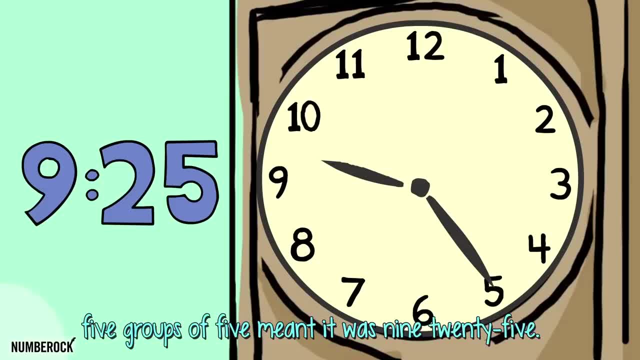 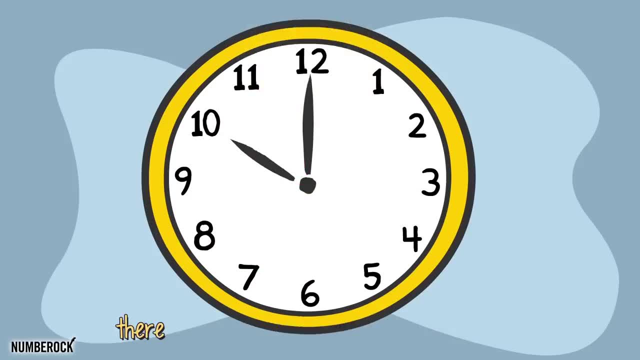 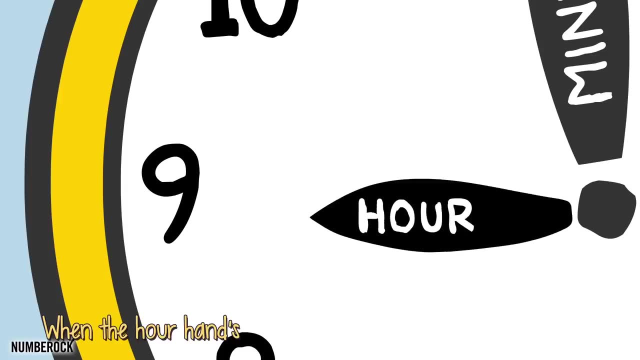 Five groups of five meant it was 925.. Oh, yeah, yeah, If you can skip down by five until times 12, there will be no time that you cannot tell. Cannot tell When the hour hands on a number and the minute hands. 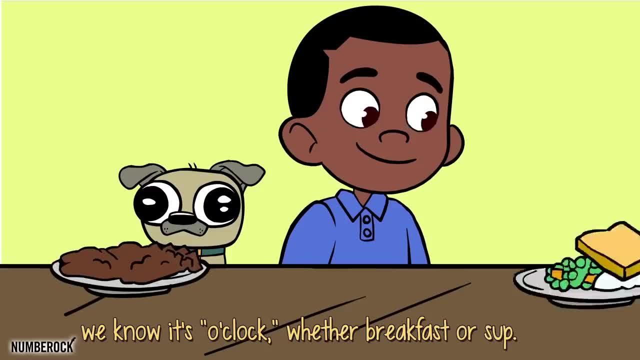 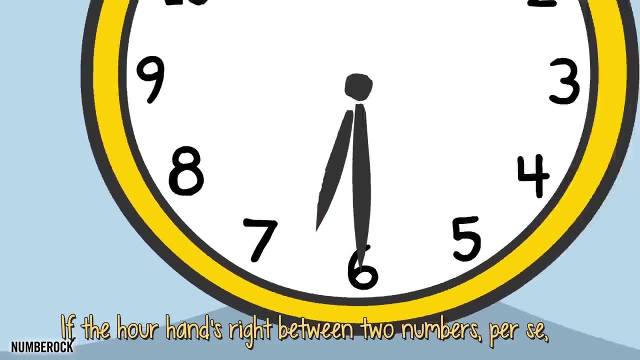 Up. we know it's o'clock where the bread was sourced up. Oh, yeah, yeah, If the hour hands right between two numbers, per say it's half past an hour or 6.30 that day, Yes, it is. 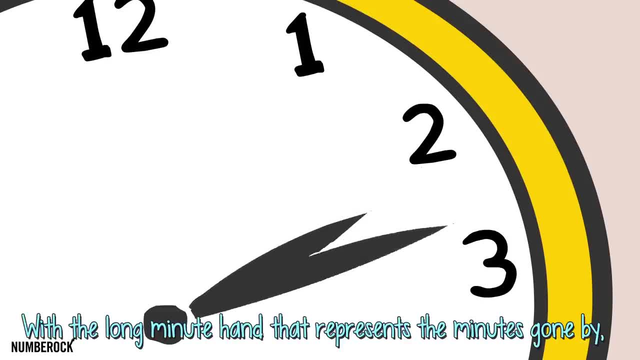 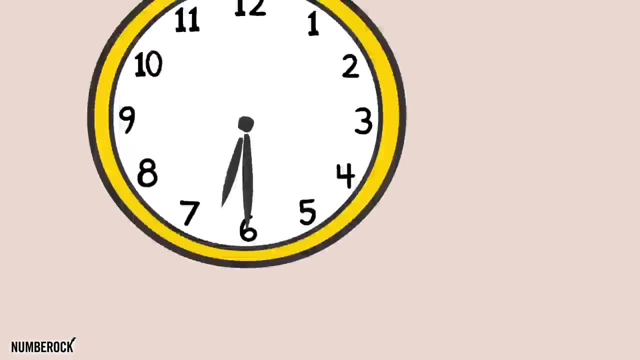 With the long minute hand that represents the minutes gone by, it's easy to tell time and you soon see why Each number on the clock is four minutes, Five minutes in it. If you skip, count by five, you'll tell the time. 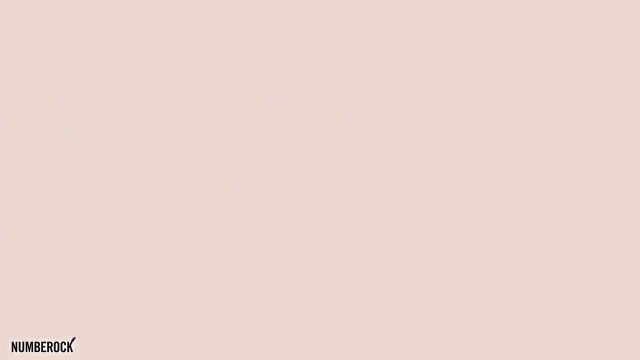 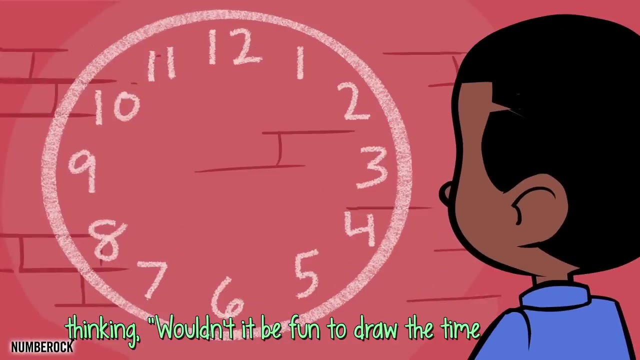 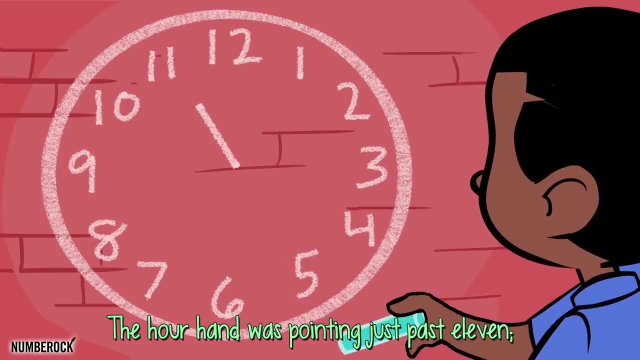 Nicky, it's split. After an hour of playing. I took my sidewalk chalk Thinking wouldn't it be fun to draw the time on a clock. Hmm, oh yeah, The hour hand was pointing just past 11.. Two groups of five was 10, so it was 11-10.. 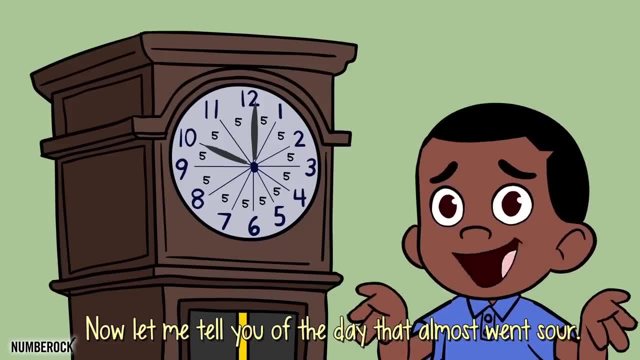 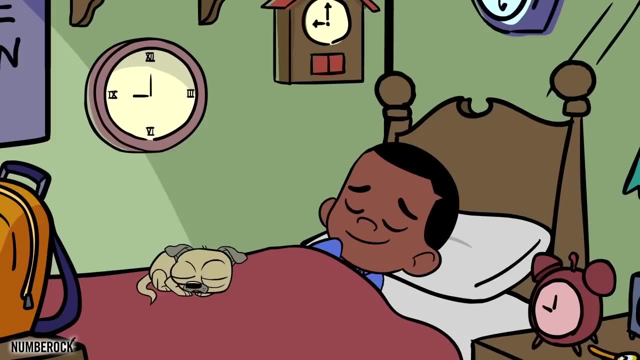 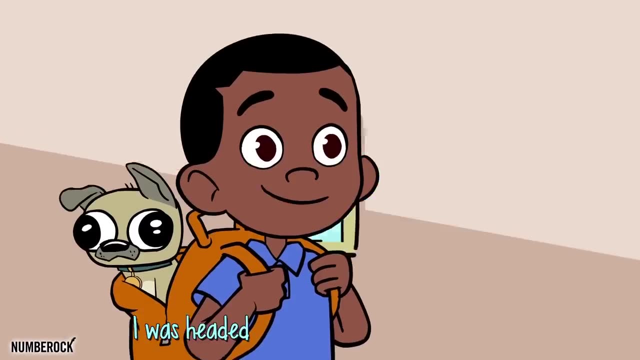 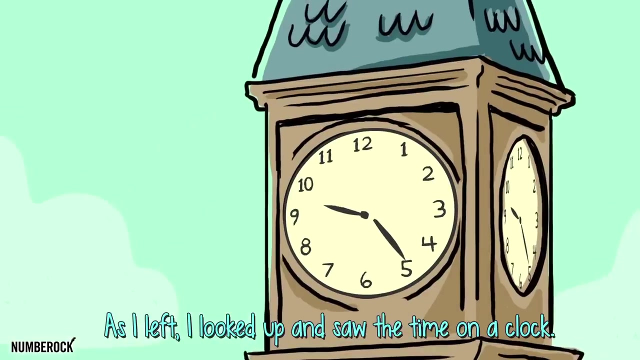 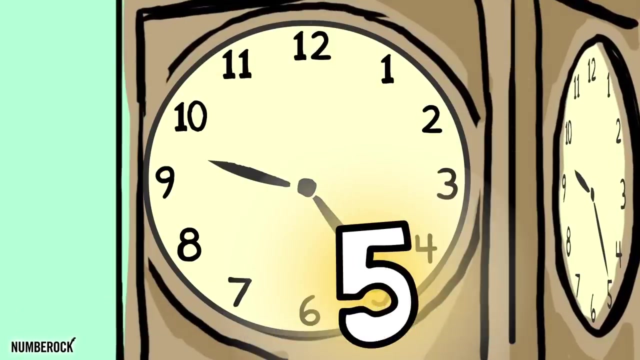 Now let me tell you of the day that almost went sour. Oh yeah, I was headed to the park. I decided to walk As I left. I looked around, I looked up and saw the time on the clock. The shorthand was after nine. then one, two, three, four, five. 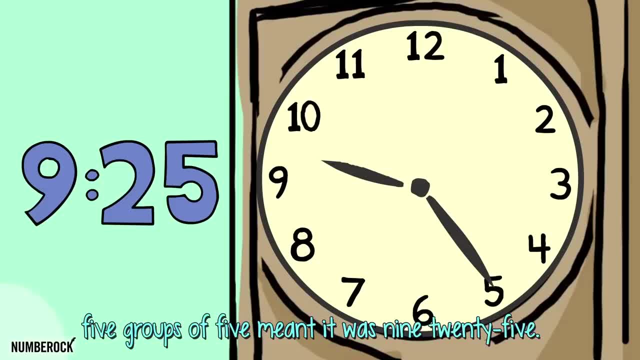 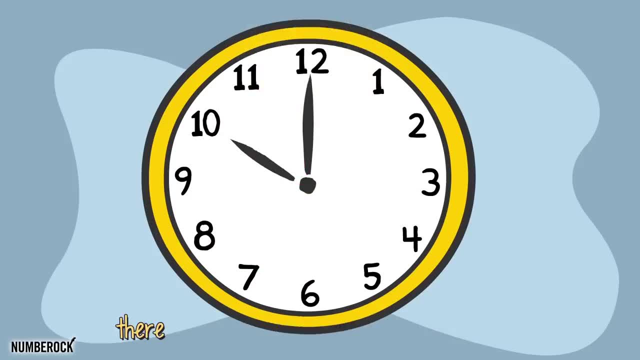 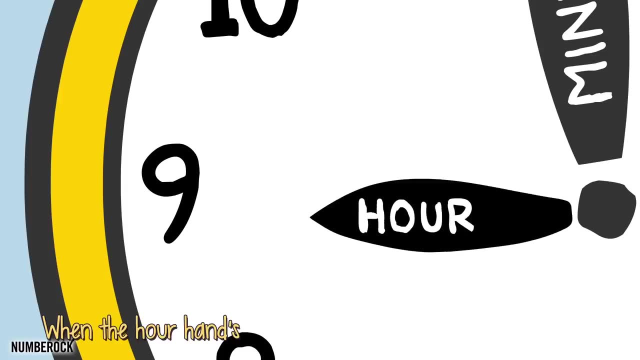 Five groups of five meant it was 925.. Oh, yeah, yeah, If you can skip down by five until times 12, there will be no time that you cannot tell. Cannot tell When the hour hands on a number and the minute hands. 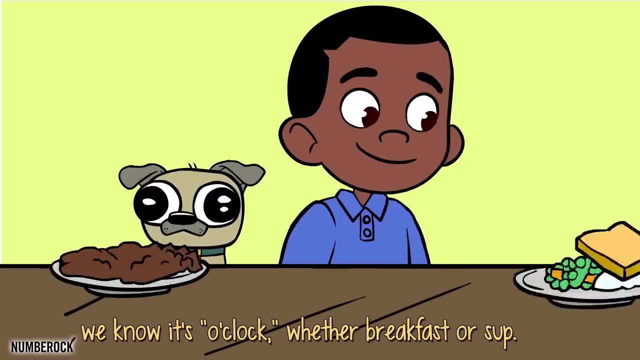 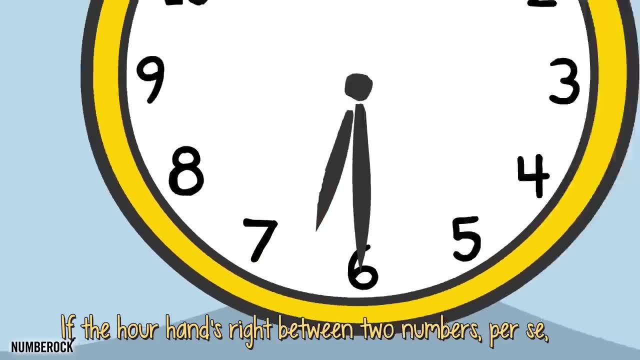 Up. we know it's o'clock where the bread was sourced up. Oh, yeah, yeah, If the hour hands right between two numbers, per say it's half past an hour or 6.30 that day, Yes, it is. 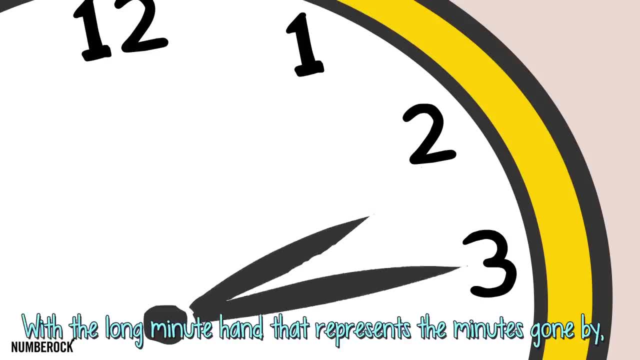 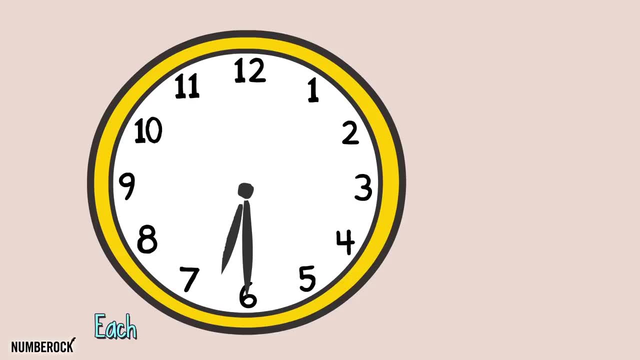 With the long minute hand that represents the minutes gone by, it's easy to tell time and you soon see why Each number on the clock is four, It's five minutes in it. If you skip, count by five, you'll tell the time. 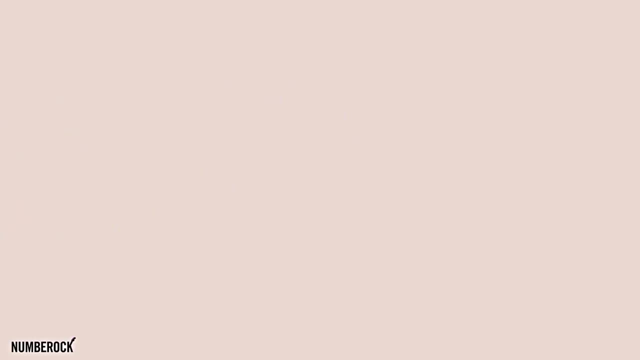 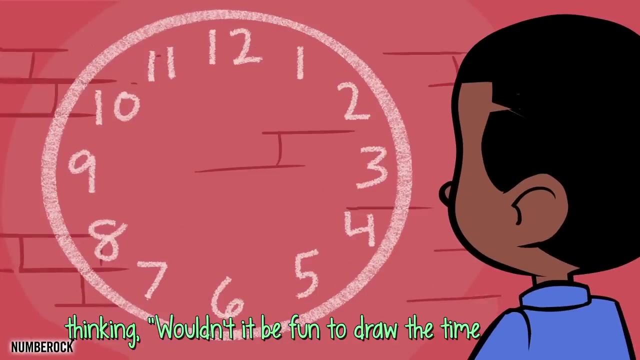 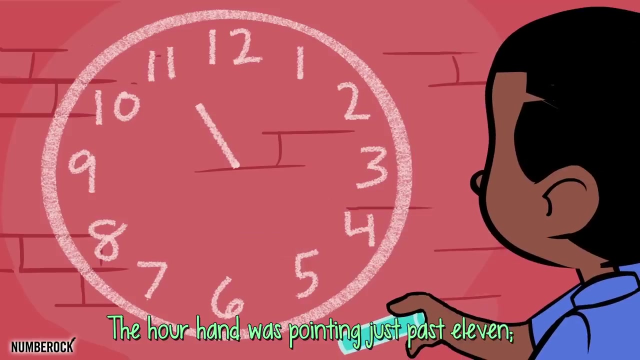 Likety split. Yeah, yeah, After an hour of playing I took my sidewalk chalk Thinking: wouldn't it be fun to draw the time on a clock Ten times, ten times, ten times. The hour hand was pointing just past 11.. 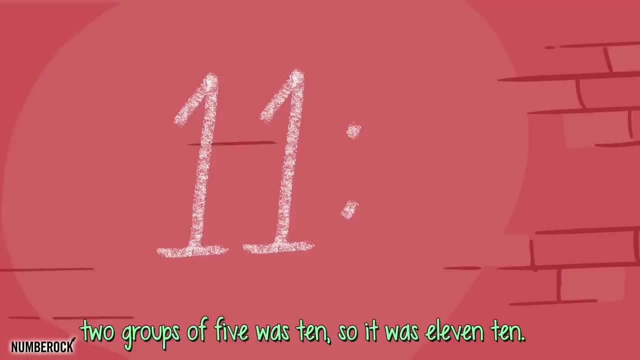 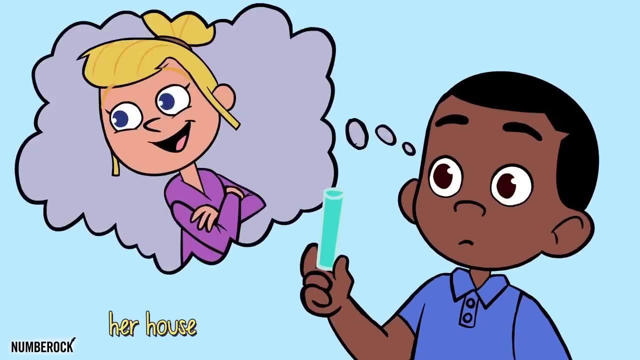 Two groups of five was ten, so it was 11-10.. 11-10., 11-10.. I remembered I had to meet my friend Lexi. Her house was far away, so I left in a hurry. A hurry, hurry, hurry, hurry. 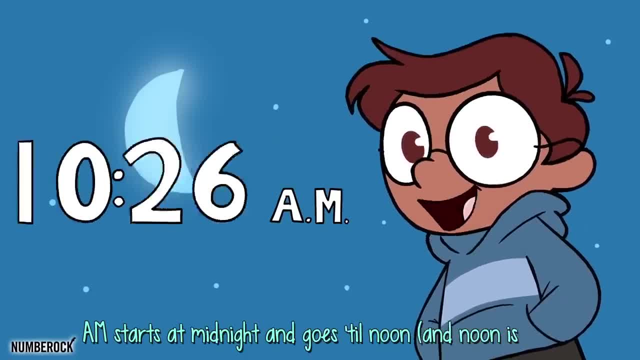 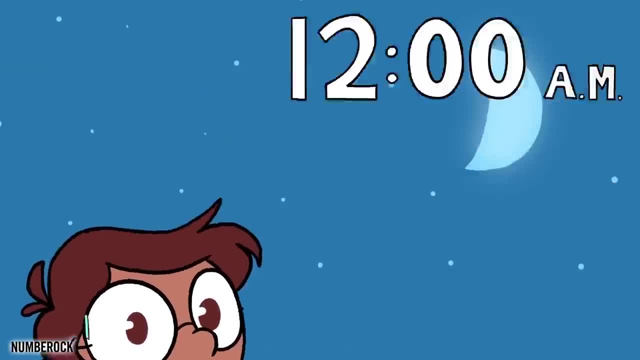 AM starts at midnight and goes till noon, and noon is 12 pm. PM starts at noon and goes till midnight's moon and midnight's 12 am. I got to Lexi's door and then rapped, knock, knock. 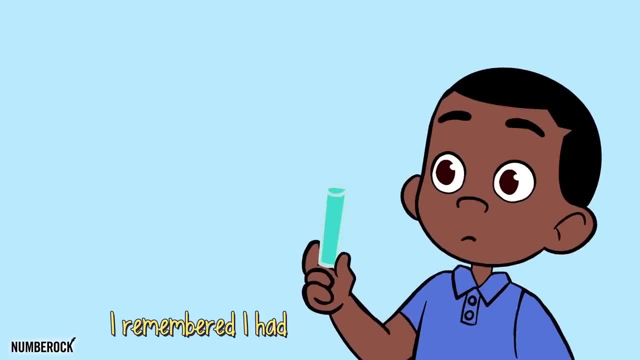 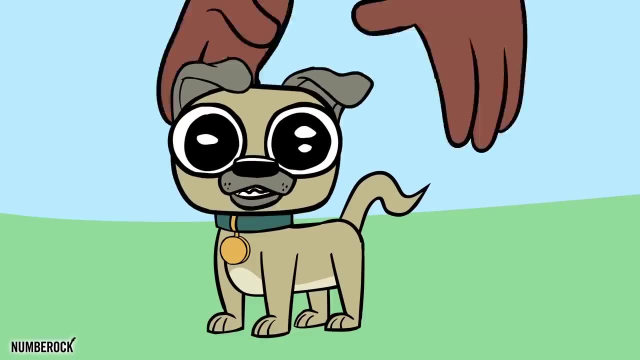 11-10., 11-10., 11-10., 11-10., 11-10., 11-10.. I remembered I had to meet my friend Lexi. Her house was far away, so I left in a hurry. 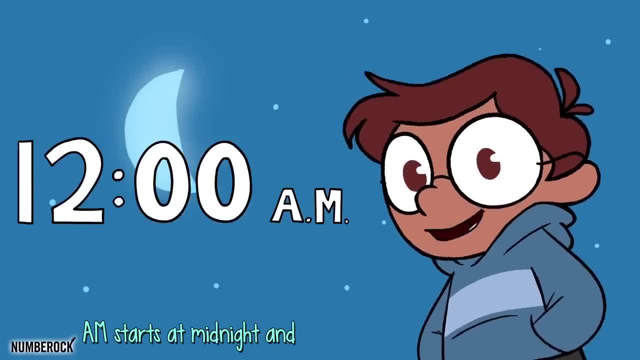 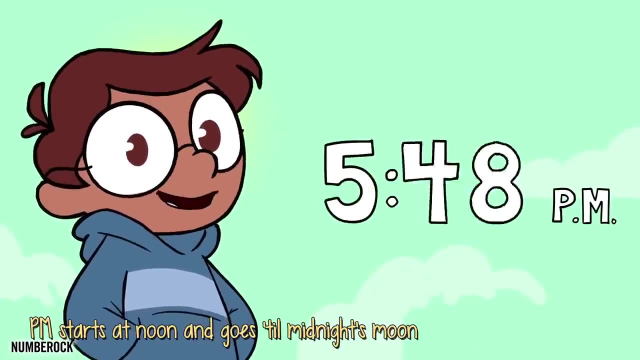 A hurry, A hurry. A-M starts at midnight and goes till noon, and noon is 12 pm. P-M starts at noon and goes till midnight, smooth, and midnight is 12 am. I got to Lexi's door and then rapped. 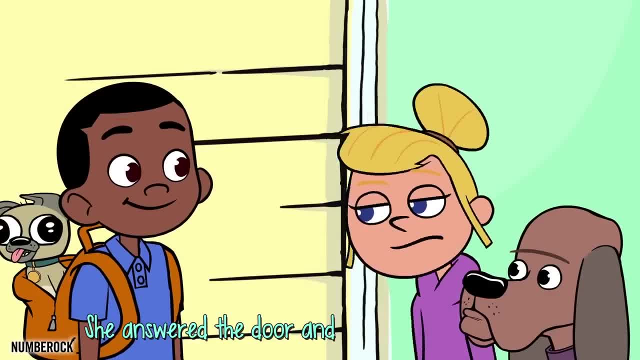 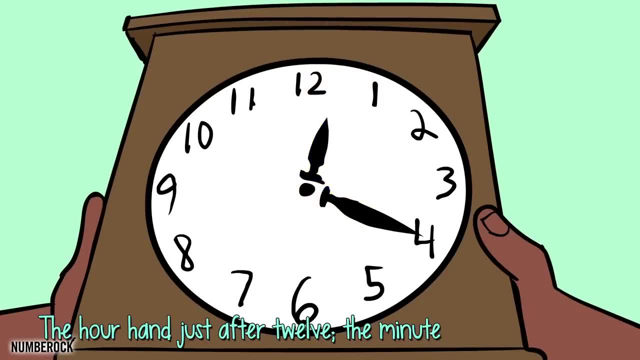 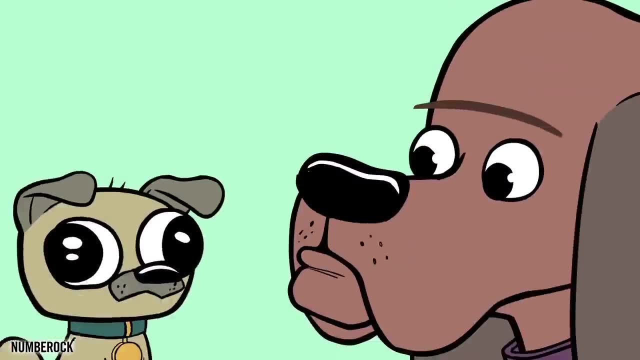 Knock Knock. She entered the door and was pointing to the clock, Tick Tock, Tick Tock. The hour hand just after twelve. the minute hand at the four, Four times five was twenty minutes. her foot tapped on the floor, The time was twelve twenty and she looked annoyed. 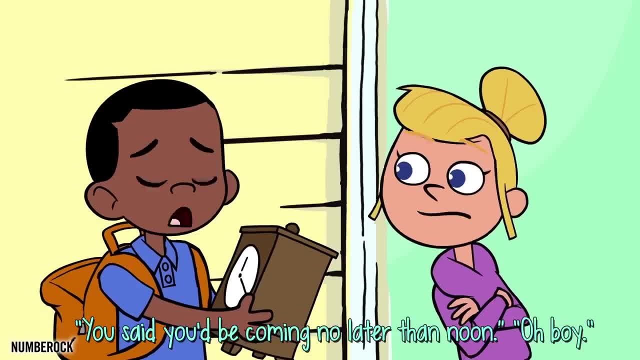 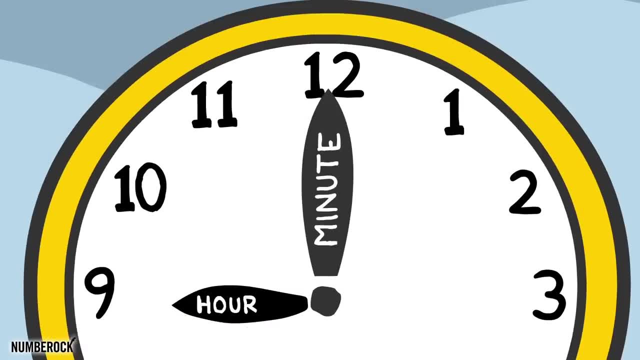 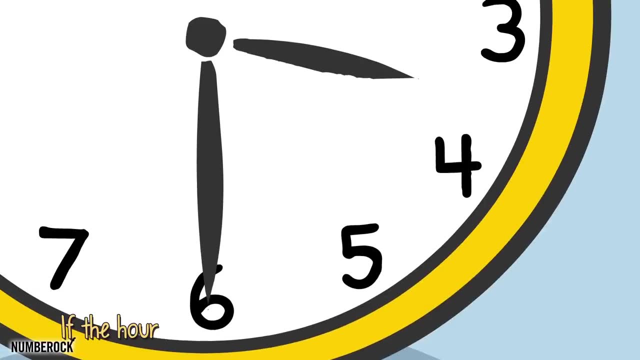 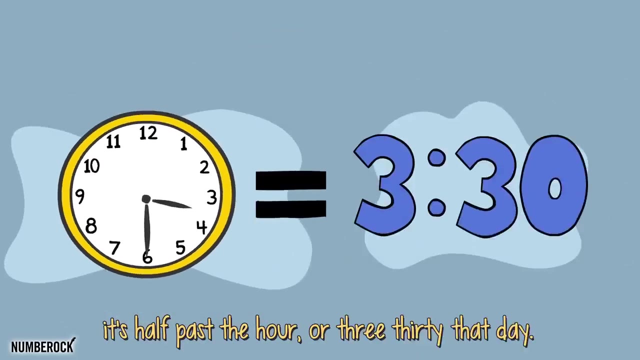 You said you'd be coming no later than noon. Oh boy, When the hour hands on a number and the minute hands up, We know it's o'clock where the breakfast's ours up. If the hour hand's right between two numbers, per say, It's half past an hour. all three thirty bad days. 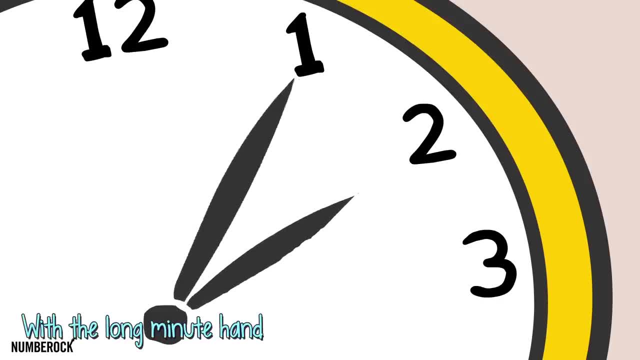 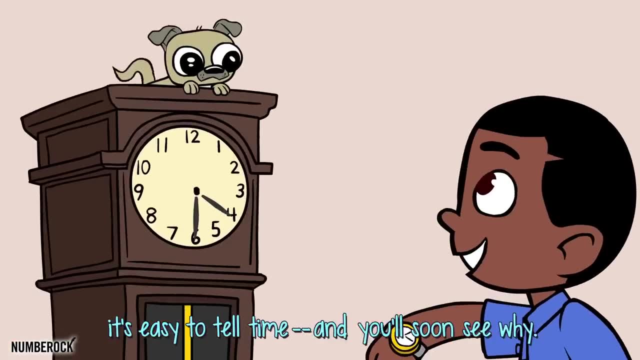 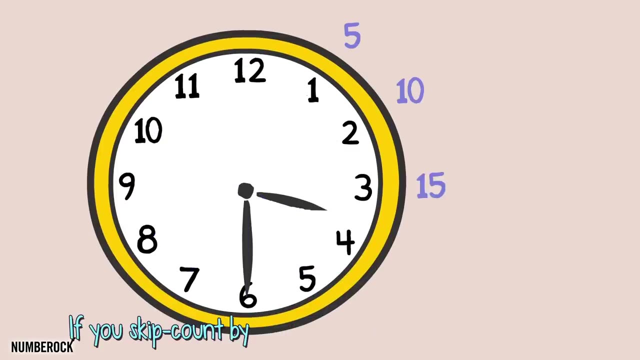 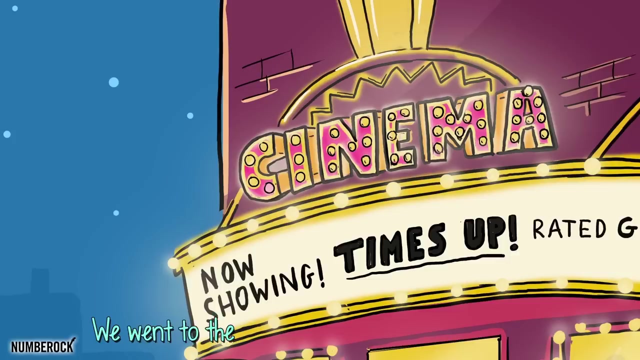 With the long minute hand that represents the minutes gone by, It's easy to tell time, and you'll soon see why Each number on the clock has five minutes in it. If you skip, count by five, you'll tell the time. Oh boy, We went to the movies and they bought us two tickets. 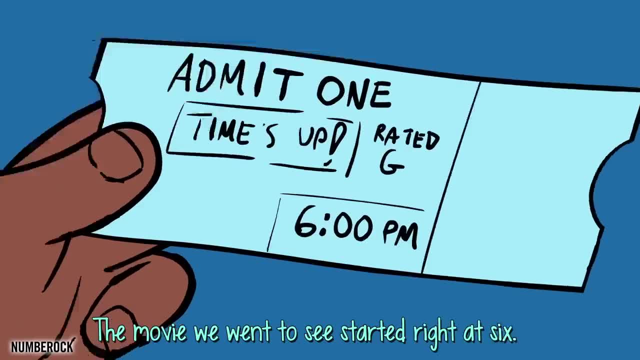 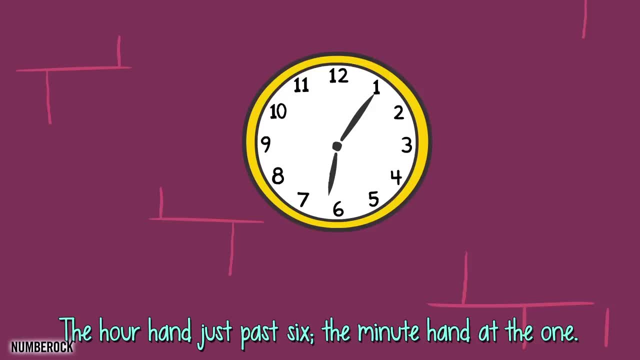 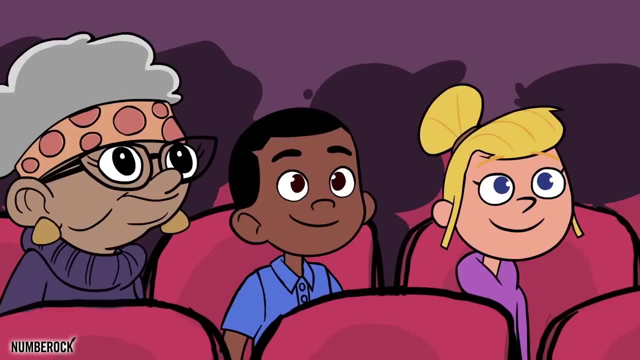 The movie we went to see started right at six The hour hand. just past six the minute hand at the one, She said it's six o' five, aren't we late? And I was like, oh yeah. When we finally got our seats she told me I was cute. 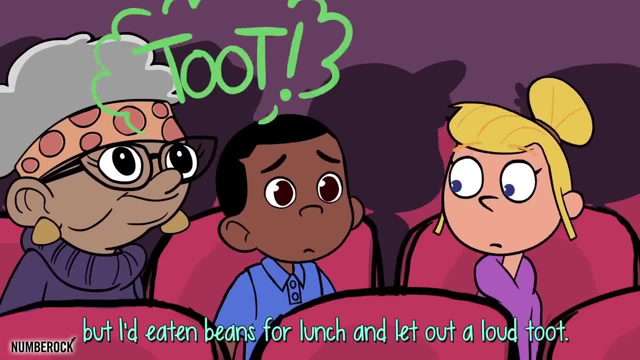 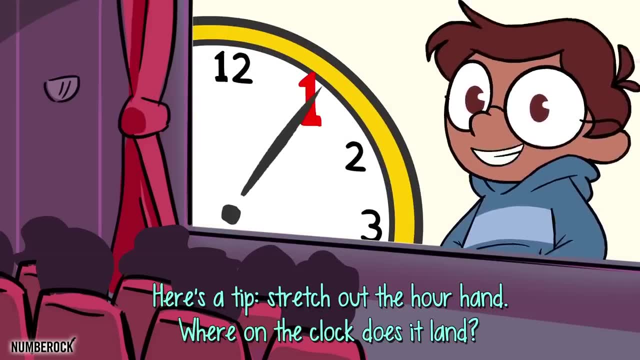 But I'd eaten before I got home. Oh boy, We ate some beans for lunch and let out a loud toot. Oh, no, no, no. Here's a tip stretch of the hour hand We're on. the clock doesn't land. The last number it went by tells you the hour of time. 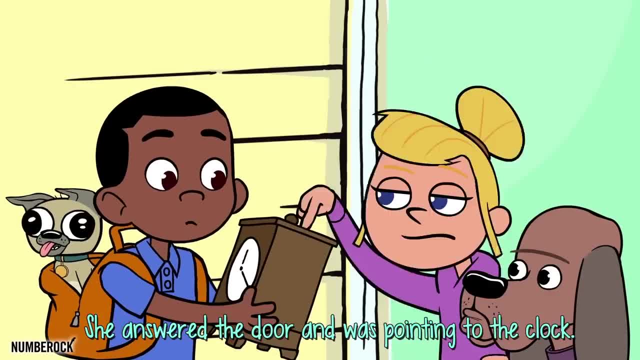 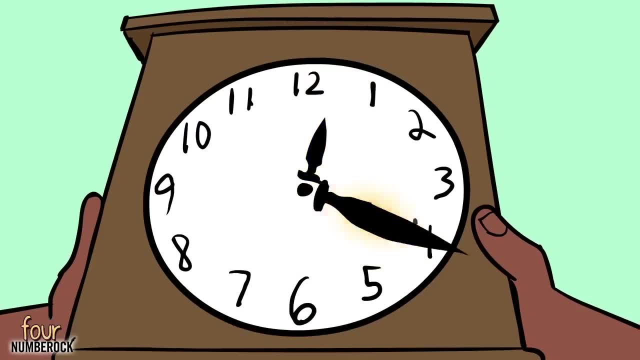 She entered the door and was pointing to the clock, Tick-tock, Tick-tock, Tick-tock. The hour hand just sat at 12, the minute hand at the 4.. Four times five was 20 minutes. her foot tapped on the floor. 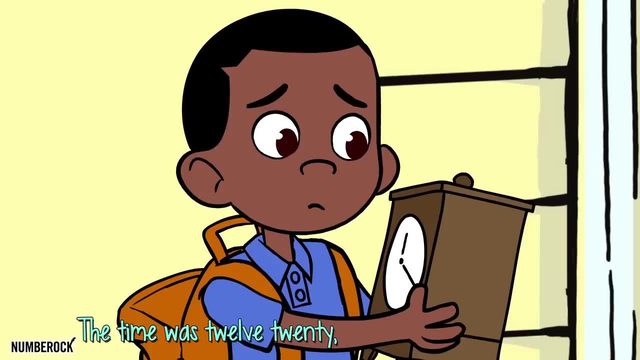 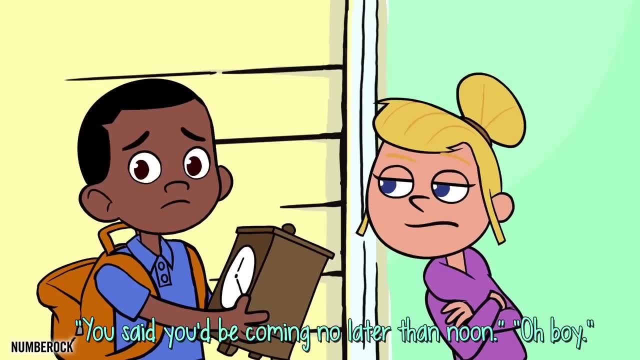 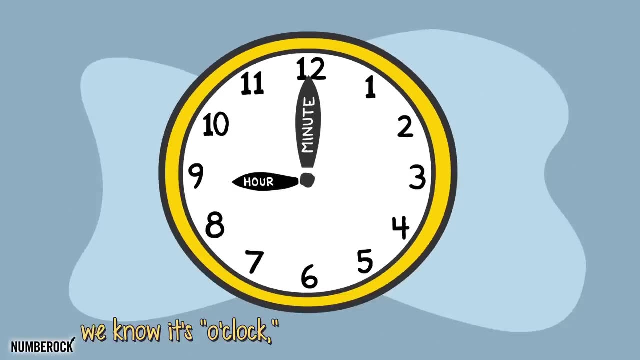 Oh yeah, yeah, The time was 12-20, and she looked annoyed. You said you'd be coming no later than noon. Oh boy, When the hour hands on a number and the minute hands up, we know it's o'clock. 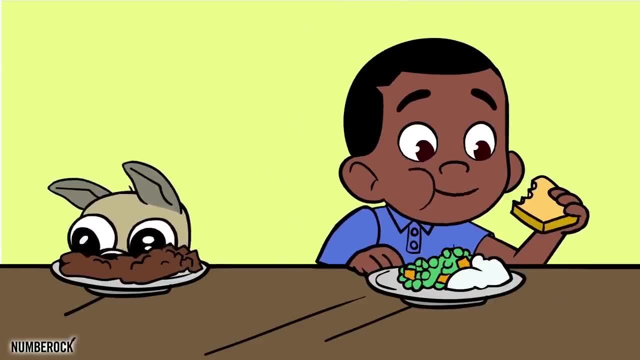 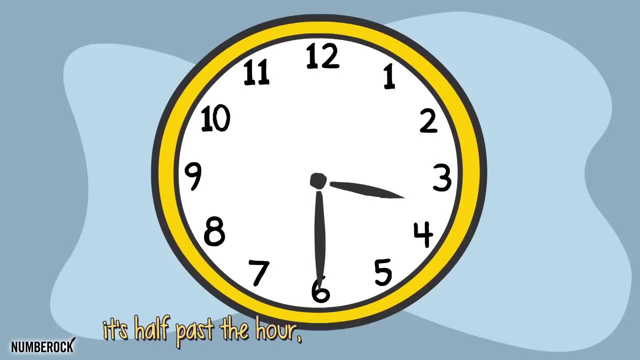 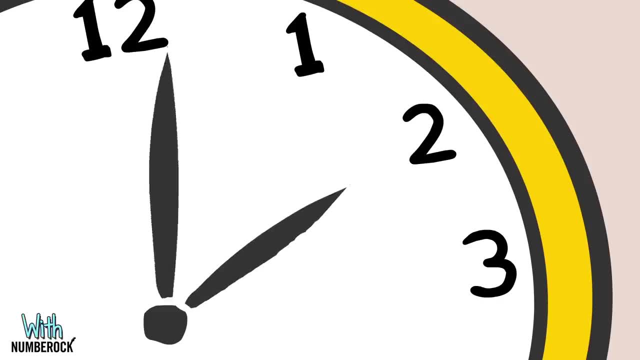 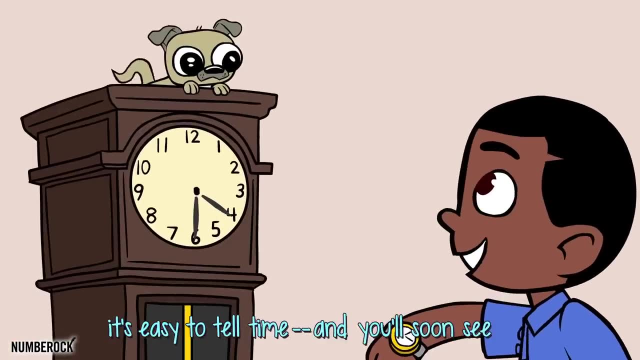 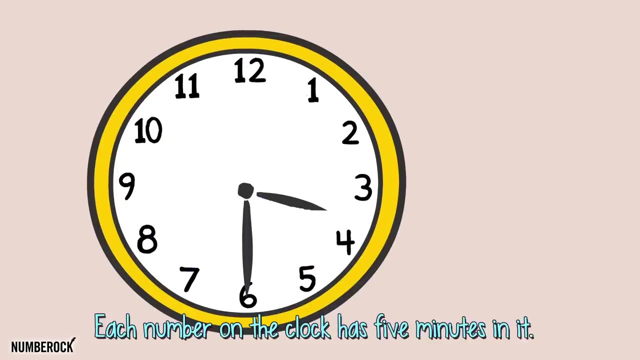 day. It isn't easy. it isn't easy With the long minute hand that represents the minutes gone by. it's easy to tell time and you'll soon see why. Each number on the clock has five minutes in it. If you skip, count by five, you'll tell. it's so easy. you'll soon see why. 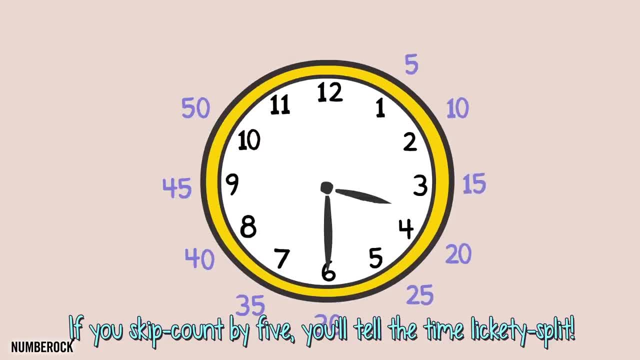 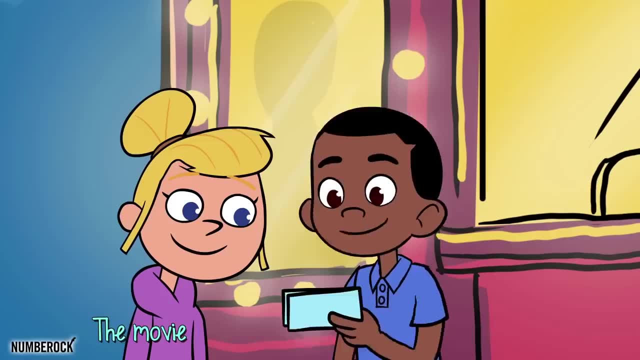 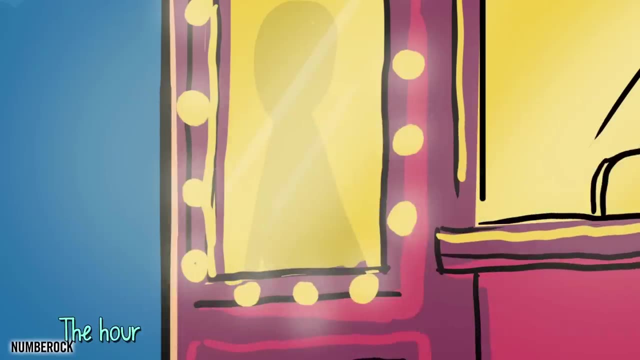 If you skip, count by five you'll tell it's so easy. you'll soon see why We went to the movies and they bought us two tickets. The movie we went to see started right at six. The hour hand just passed six. the minute hand at the one. 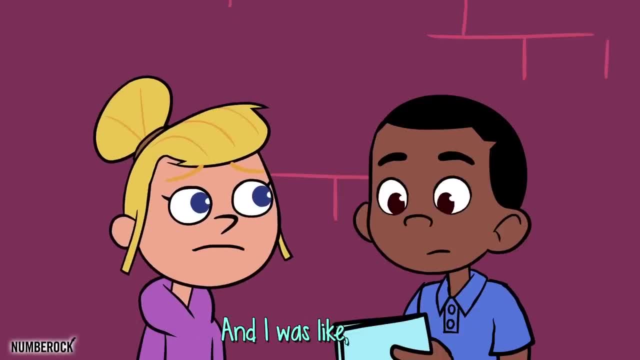 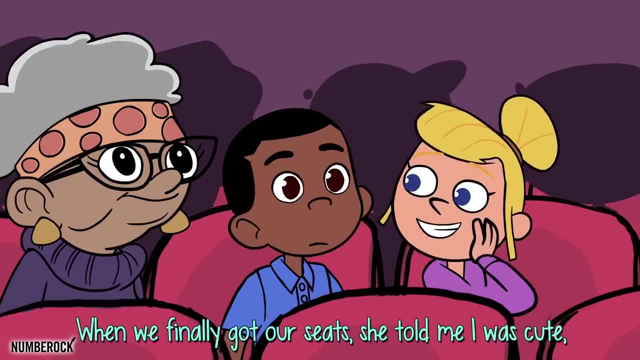 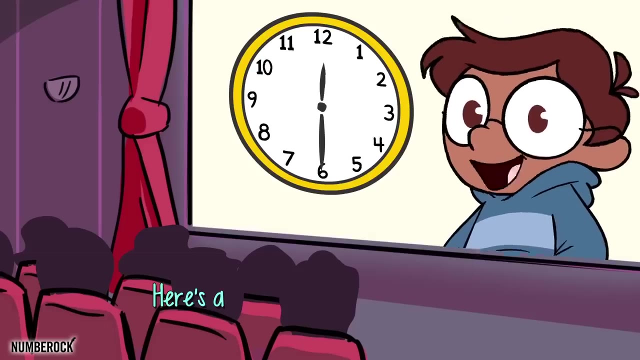 She said it's 6.05, aren't we late? And I was like, oh yeah. When we finally got a seat, she told me I was cute, But I'd eaten beans for lunch and let out a loud toot. Here's a tip. stretch of the hour hand. 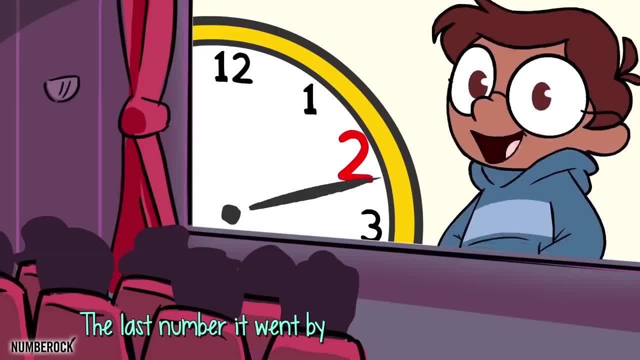 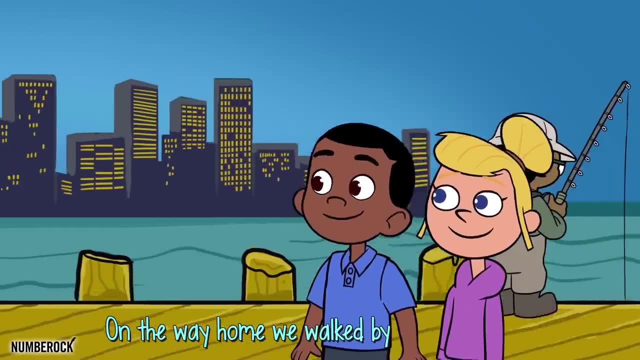 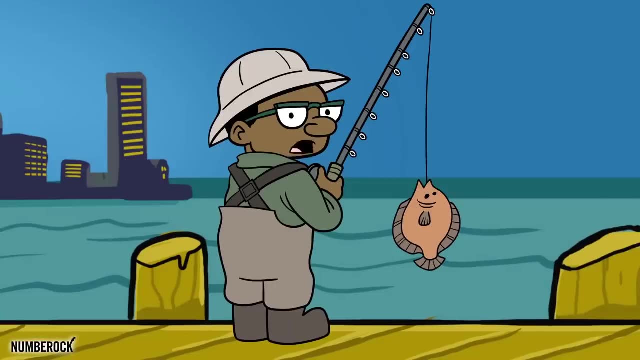 We're on, the clock doesn't land. The last number it went by tells you the hour of time. On the way home, we walked by the fishing dock. We looked up and saw that it was now eight o'clock. Oh yeah, My, my, my. 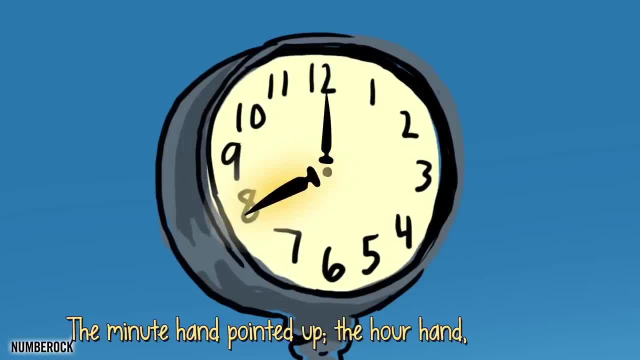 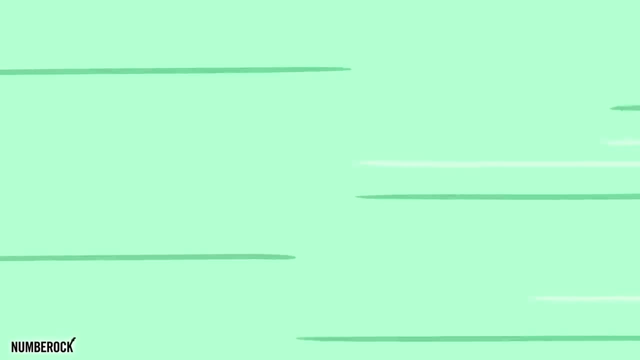 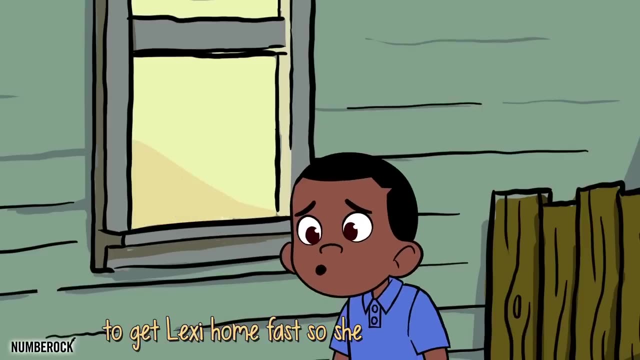 The minute hand pointed up the hour hand at the eight She said: my curfew's quarter after eight. Oh great, That's 8.15. Oh, no, no. So we went off in a hurry, hurry. We ran, we bounded To get Lexi home fast so she wouldn't be grounded.